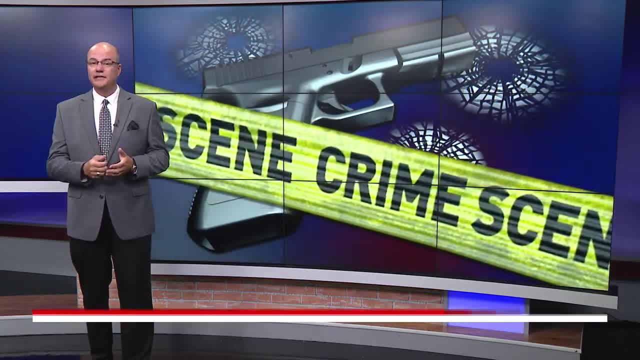 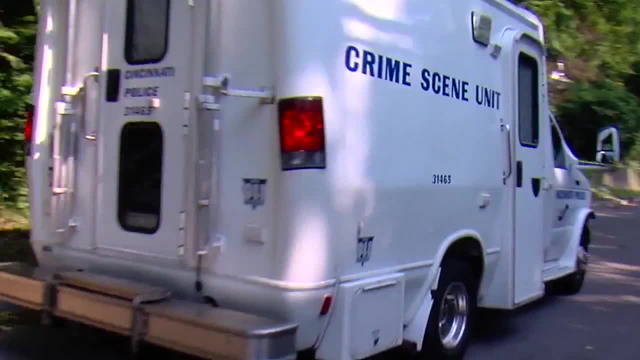 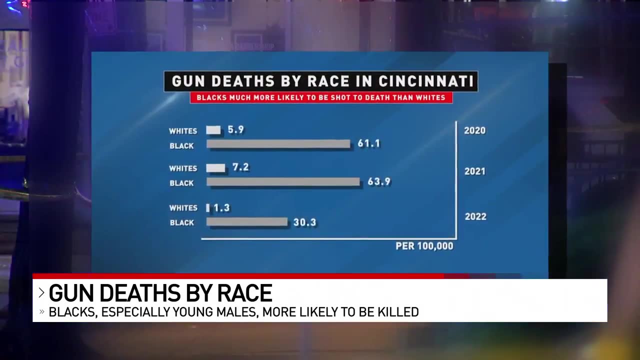 We've seen two years of record homicide numbers and gun violence in the city And, according to my data analysis, one community and age group is by far suffering the most. Overall, the gun death rate for blacks far exceeded that for whites in Cincinnati in the last few years, as you can see here. 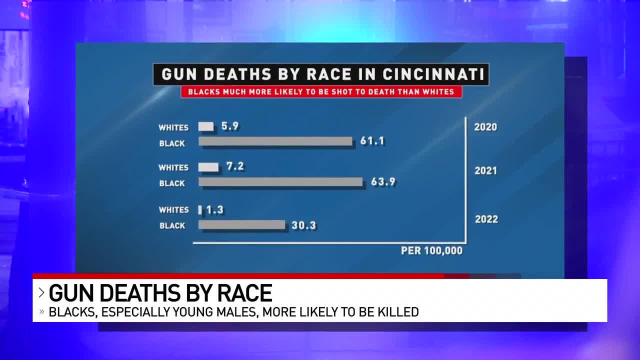 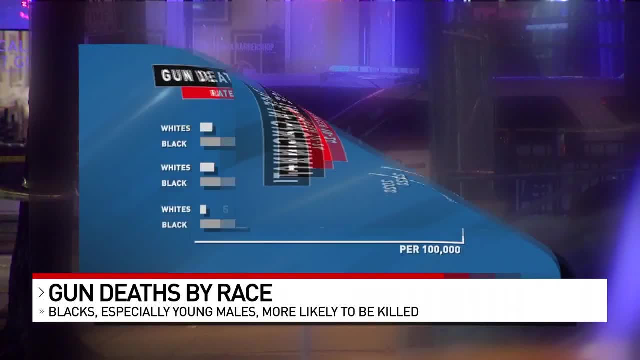 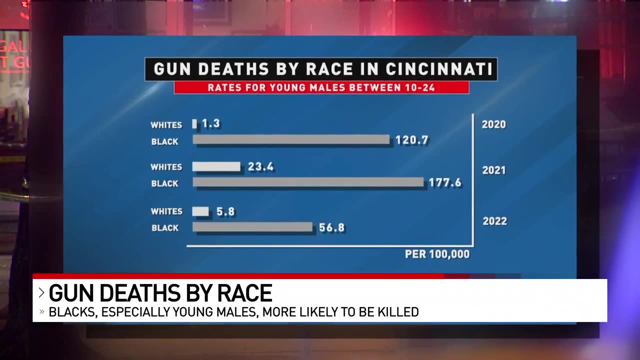 In some cases 40 times higher. The numbers are provided by the Cincinnati Police Department, cross-matched with the most recent census population estimates. Compare that to the rates for youths- Young males ages 10 to 24.. In May, the CDC reported the rate for blacks in this age group was 21 times higher than whites in 2020 alone. 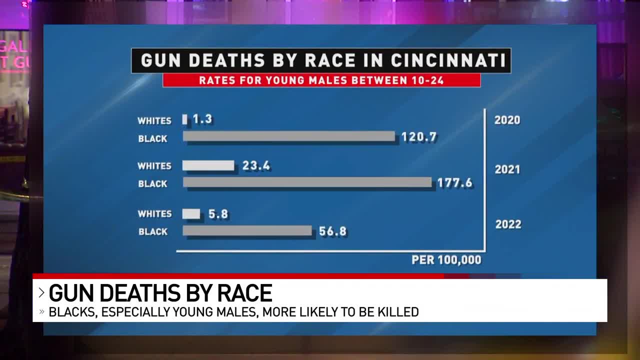 In Cincinnati that year it was nearly 120 times higher, meaning a young black male was more than 100 times more likely to die from gunfire than a young white male, And last year the gun death rate for young black males here more than doubled the national rate. 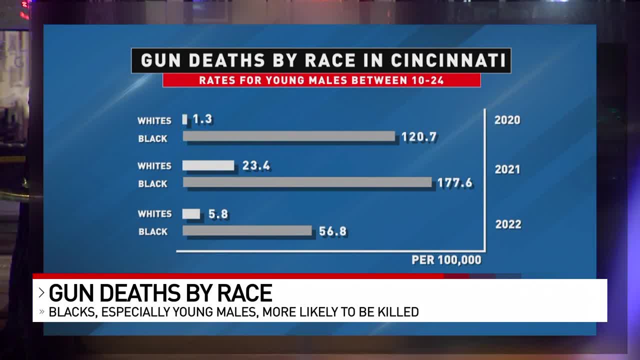 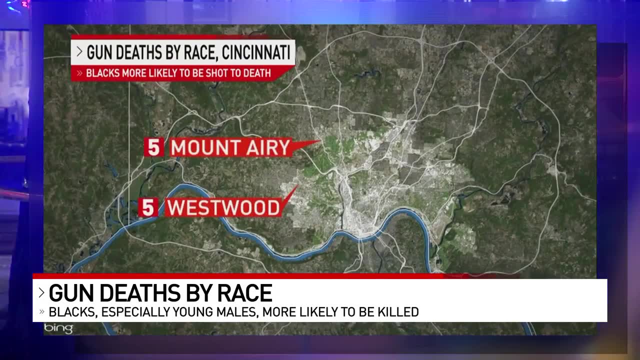 So far, 2022 also shows a wide gap between blacks and whites in this age group, And this year the most killings have occurred in these neighborhoods. Mount Airy and Westwood have had five homicides, while three people have been murdered in Northside, Bond Hill and the West End. 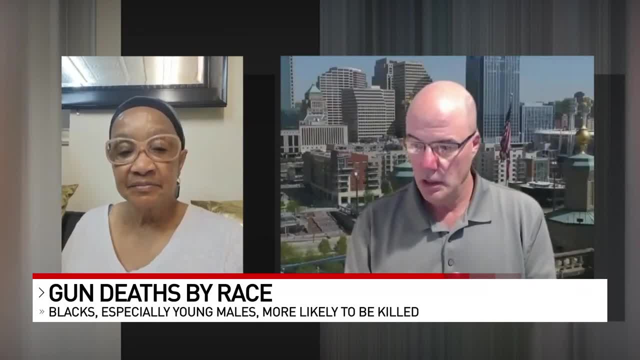 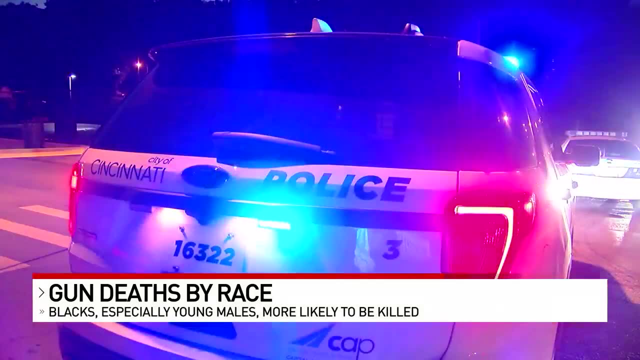 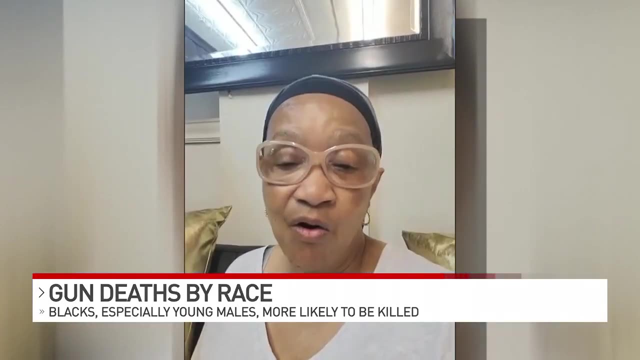 Hope Dudley founded You Speak For Me after her son died in a shooting in 2007.. The organization advocates for families of gun violence and for unsolved murders, as her son's killer has never been arrested. Guns are everywhere, And how are they getting in our community? 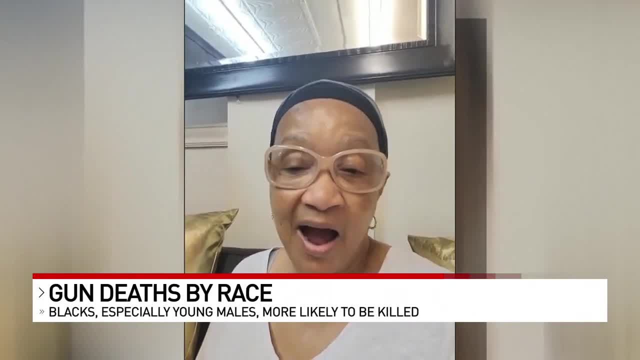 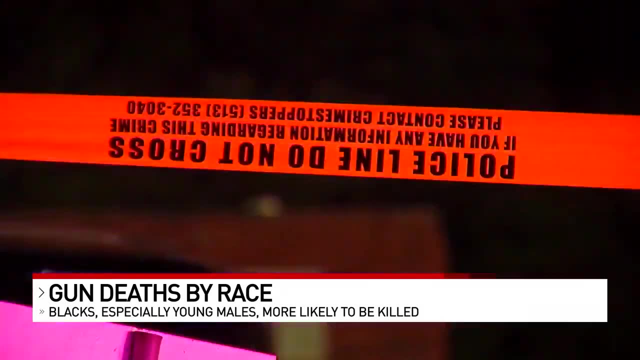 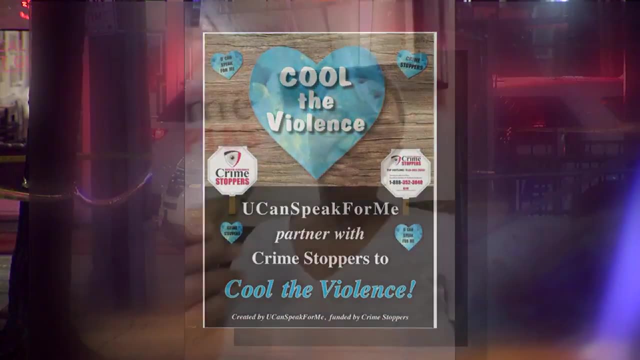 Because if a person has been arrested, I've solved for a homicide, They've had a felony, so how were they able to get the guns? This week, Dudley and Crime Stoppers launched a new campaign called Cool the Violence- handing out hand fans to raise awareness and possibly reduce the number of victims. 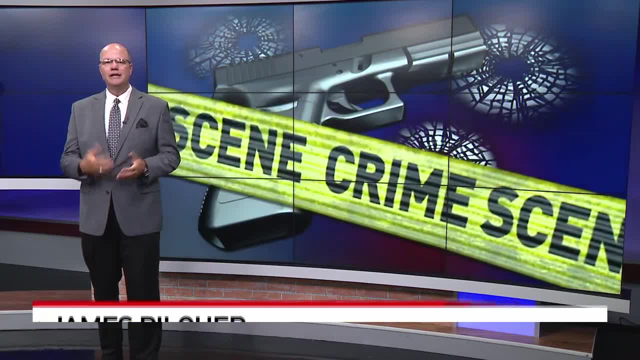 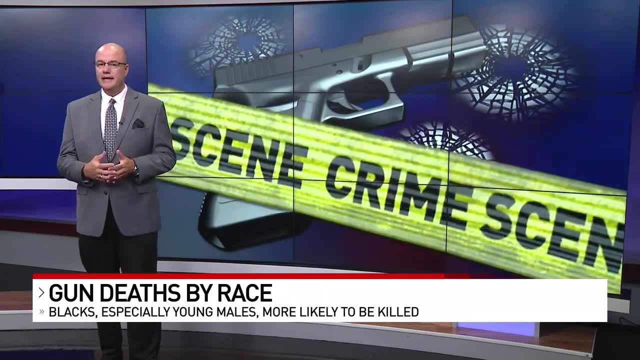 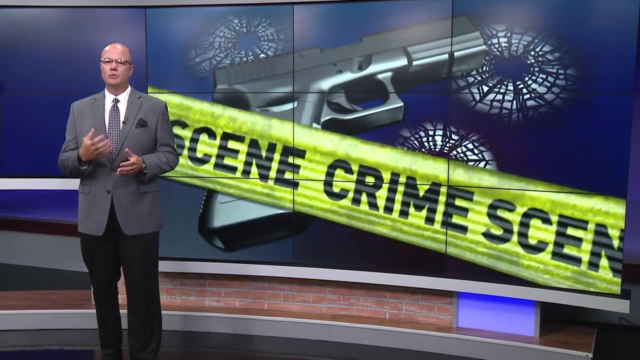 Now I asked for interviews with Cincinnati Mayor Aftab Pureval, City Manager John Kerp and someone from the Cincinnati Police Department. The mayor is out of town and not available and I did not hear back from CPD. Mr Kerp says our questions and data are definitely worth exploring, but that it's a complex issue and he wants to take some time before giving a response.